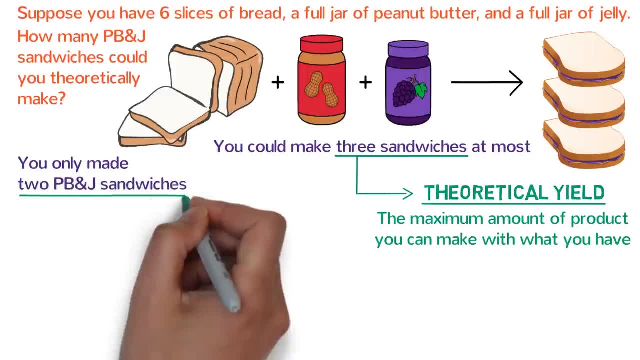 you only made two peanut butter and jelly sandwiches. That is what we call the actual yield. in chemistry, It is the amount of product that is actually made and collected. Chemists often like to compare the actual and theoretical yields, and they do so by calculating. 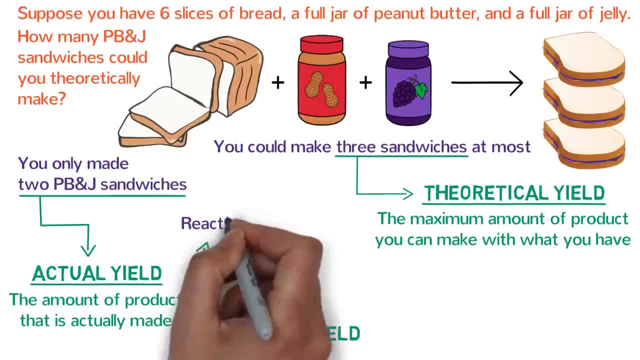 the percent yield, which is more or less a measure of reaction efficiency. The percent yield tells you how well your reaction worked. It is defined as the actual yield divided by the theoretical yield, all multiplied by 100 in order to convert it to a percentage, We can calculate the percent. 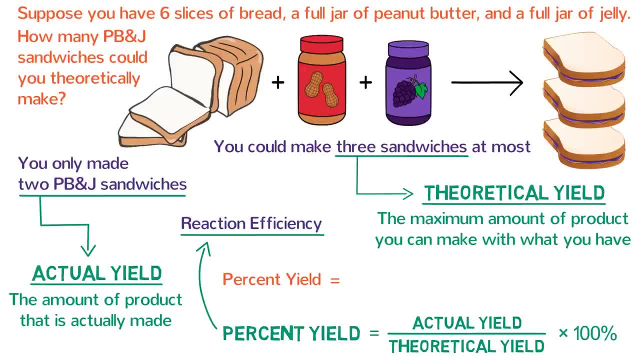 yield of our peanut butter and jelly sandwiches by dividing the actual yield of two sandwiches by the three sandwiches, After multiplying that by 100, we see that the percent yield of this experiment is 67%. Okay, now we're ready for calculating the percent yield of a real chemical reaction. 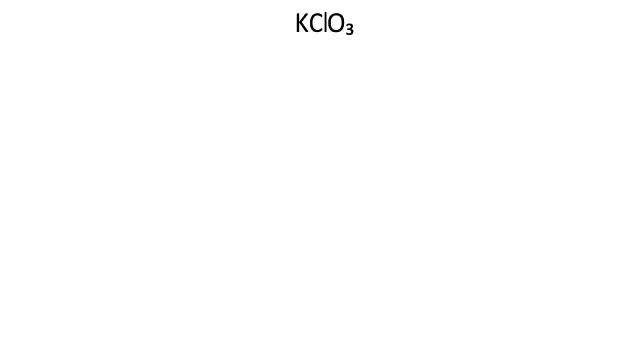 Consider the decomposition of potassium chlorate. Like other metal chlorates, it will decompose when heated, and the products of its decomposition are potassium chloride and oxygen gas. You can form this reaction in the lab in order to make oxygen, but you need to be careful because small 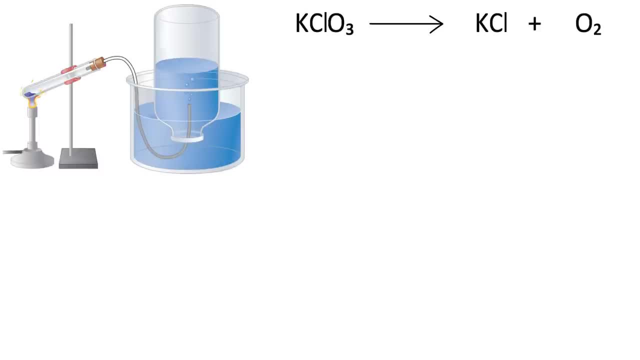 amounts of impurities or exposing potassium chloride to organic compounds such as plastics, grease or rubber could result in a dangerous explosion. In order to speed up this reaction, the catalyst manganese oxide is typically added. Catalysts are often written below the reaction arrow. Remember that a catalyst speeds up a reaction without being changed itself. The 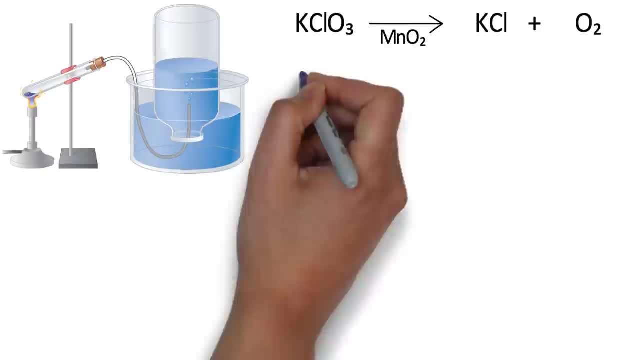 manganese oxide is not really part of the reaction, so we will ignore MnO2 for all of our stoichiometry equations. As it is written, the reaction is not balanced, so let's go ahead and fix that. There are three oxygens on the left side and two oxygens on the right side, so we put a 2 in front. 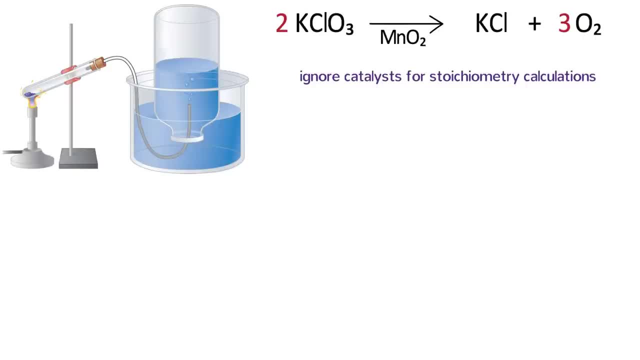 of potassium chlorate and a 3 in front of O2, to give us six oxygens on both sides. This messed up potassium and chlorine, which we can balance by writing a 2 in front of potassium chloride. Okay, now that the reaction is balanced, let's go ahead and see what the question is In the lab. 10 grams. 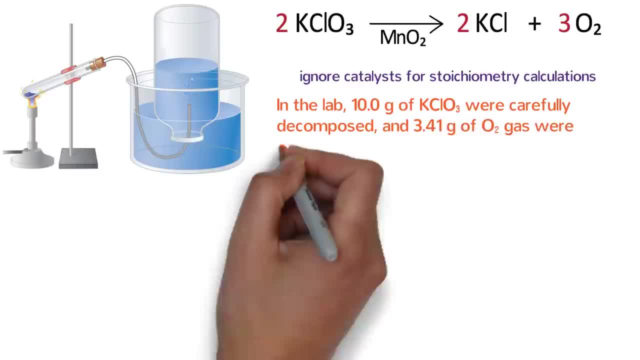 were carefully decomposed and 3.41 grams of oxygen gas were collected. What are the theoretical, actual and percent yields of the reaction? The theoretical yield is the amount of product that should be made from the amount of reactant you are starting with. So this is a grams-to-grams. 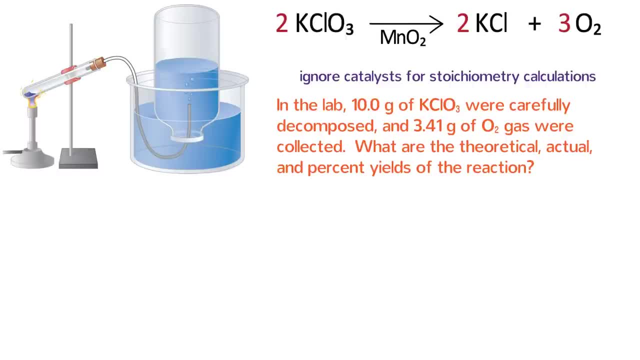 stoichiometry problem. going from the reactant to the product, We are going to need the molar masses of the chemicals, which we can solve by adding up the molar masses of the elements each one is made of. Potassium chlorate has to be added to the reactant to make the reactant Potassium chlorate. 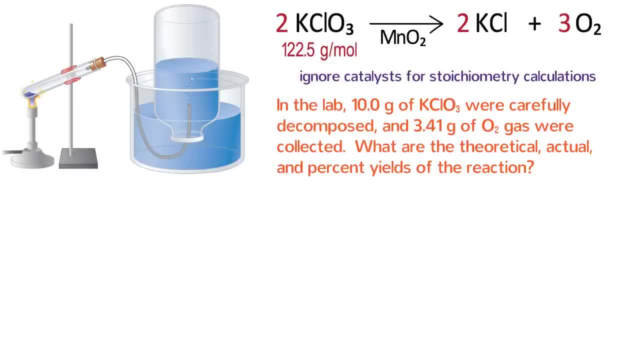 has to be added to the reactant to make the reactant. Potassium chlorate has to be added to the reactant to make the reactant. Potassium chlorate has a molar mass of 122.5 grams per mol. There are two. 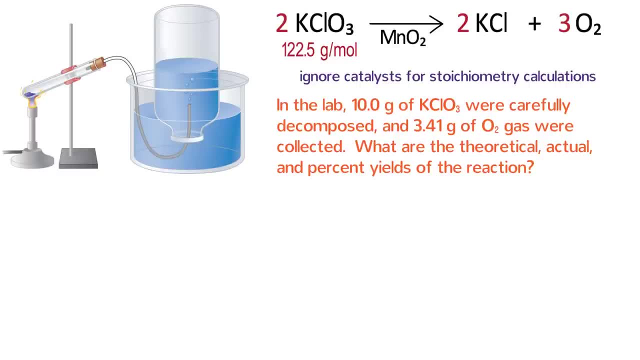 products. Which one should we solve for? Because the question tells us the amount of O2 collected. we should solve for O2, not KCl. The molar mass of O2 is 32 grams per mol. For these percent yield questions, always start your stoichiometry calculations by writing down the mass of the 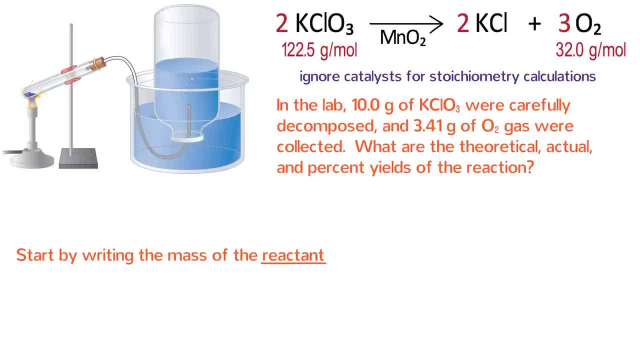 reactant, not the mass of the product. In this case, our reactant is 10 grams of potassium chlorate. Because this is a grams-to-gram stoichiometry problem, we are going to need three conversion factor fractions. As always, put one mole on the top left and the bottom right. This reminds us. 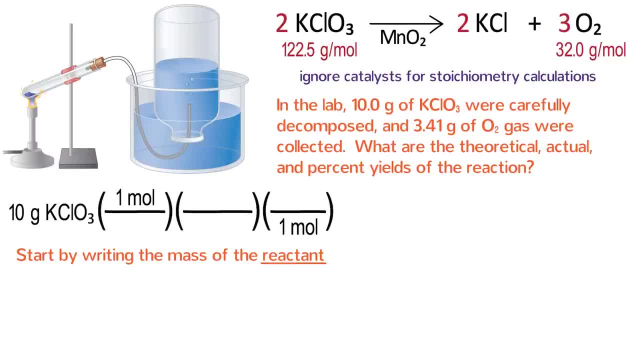 that the number on the bottom left is the mass of one mole of potassium chlorate, 122.5 grams. We also know that this is correct because grams on the top and bottom cancel each other out In the middle fraction. we always write the chemicals with their coefficients from the. 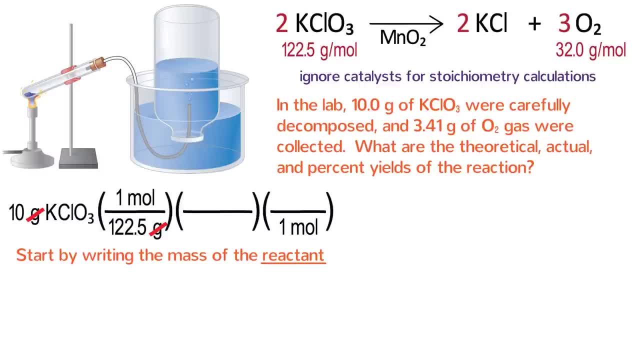 balanced reaction, Because we are starting with potassium chlorate. write 2KClO3 on the bottom. Remember that the 2 is simply the coefficient from the balanced reaction. Now, which product goes on top? Because the problem states the amount of O2 made from the. 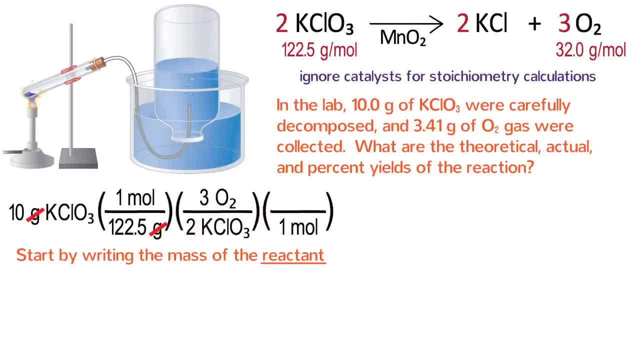 reaction. we write 3O2 on the top. Notice that potassium chlorate. on the top and bottom now cancel each other out. Lastly, on the top right goes the molar mass of O2, which is 32 grams per mole. Moles on the top and bottom cancel out. To solve this problem we need to find the 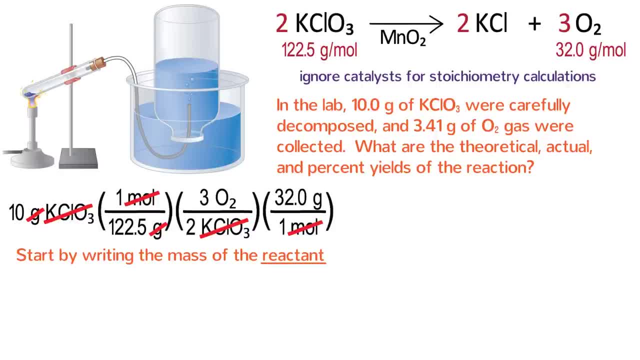 reaction. We move from left to right, always multiplying by numbers on the top of fractions and dividing by numbers on the bottom of fractions. In your calculator type, 10 divided by 122.5 times 3, divided by 2 times 32, and the answer is 3.92 grams of oxygen. 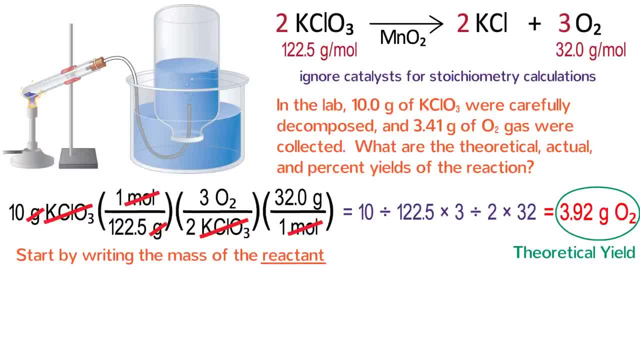 This number is the theoretical yield. It is the amount of product that we should make if everything worked perfectly. It is the maximum amount of product that we can make from the amount of reactant we started with. What is the actual yield? How much O2 did we actually make and collect? 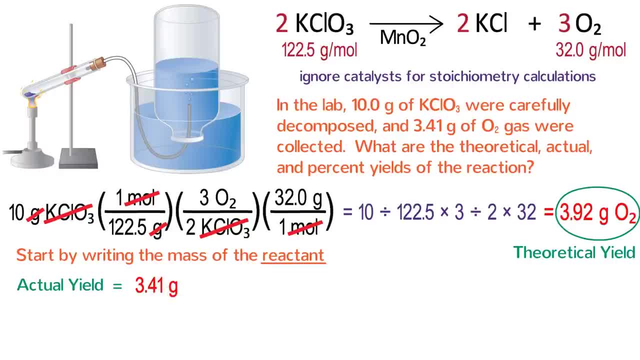 3.41 grams. Where did I get that number? Unless you are doing a lab, you always find the actual yield in the question itself. 3.41 grams of O2 gas were collected. That's the actual yield. The percent yield tells us how well the reaction worked, and we calculated by dividing the actual. 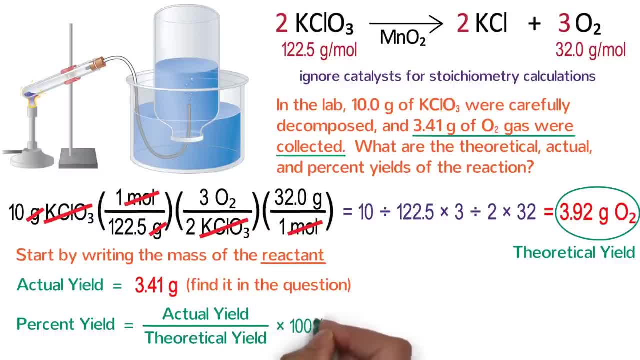 yield by the theoretical yield and multiplying the result by 1.2.. To turn it into a percent in your calculator type: 3.41 divided by 3.92 times 100, which gives us 87%, which is actually a pretty good yield as far as chemical reactions go. 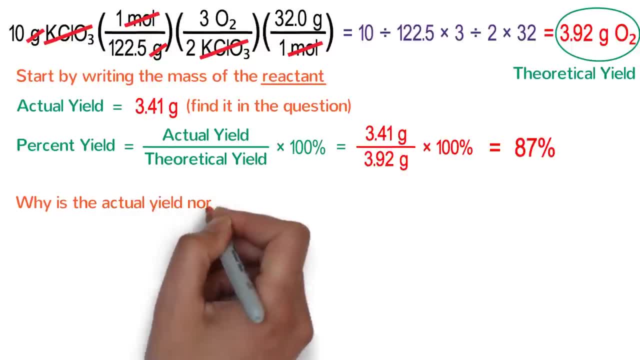 Now you might be wondering: why is the actual yield normally less than the theoretical yield? What's going on? A number of factors can contribute to this loss of product. The reaction might be incomplete, that is, the reaction can't or hasn't fully converted to product. There may be side reactions that turn the reactants or 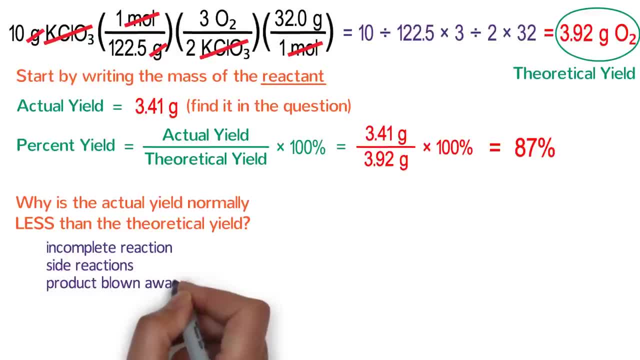 products into something different. Some of the product may get blown away or spilled. Sometimes some of the product sticks to the container and you can't get it all out. It is also possible to lose some of the product when trying to purify it. 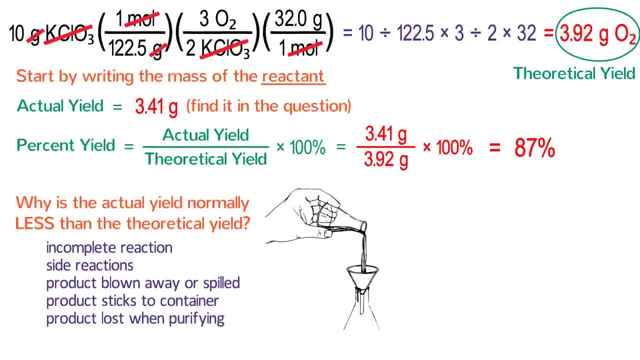 These are all normal occurrences of things that can reduce your actual and percent yields. But what if the actual yield is MORE than the theoretical yield? That is a much bigger problem, because it means that the actual yield is less than the theoretical yield and therefore you can't get it out. It's just a way to reduce what you actually have. so I'll just do a small picture. 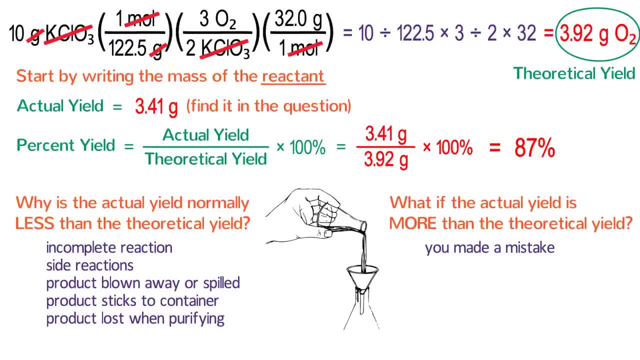 it means that you made a mistake. It is impossible to make more product than the theoretical yield. Oftentimes, this can seem to occur if the product is impure, in which case you will need to purify it or dry it. Alternatively, if the yield appears to be greater than 100%, 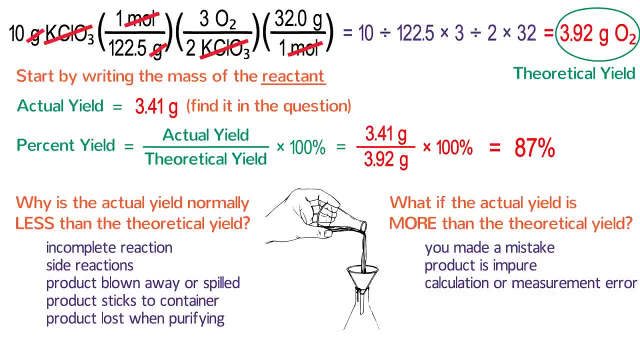 this may indicate a calculation or measurement error that you will need to go back and fix. Thanks for watching. If you found this video helpful, please give me a thumbs up. Be sure to also share any comments or questions you have below. share this video with a friend. 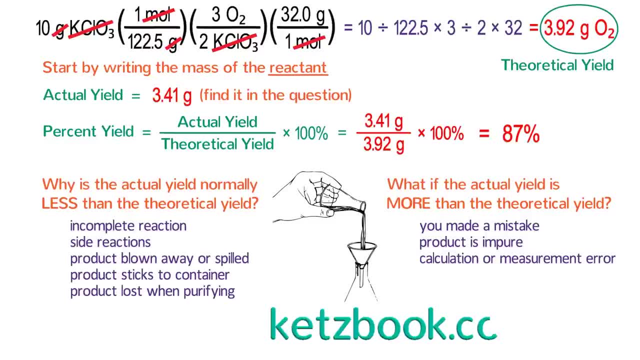 subscribe to my channel or check me out at ketsbookcom. 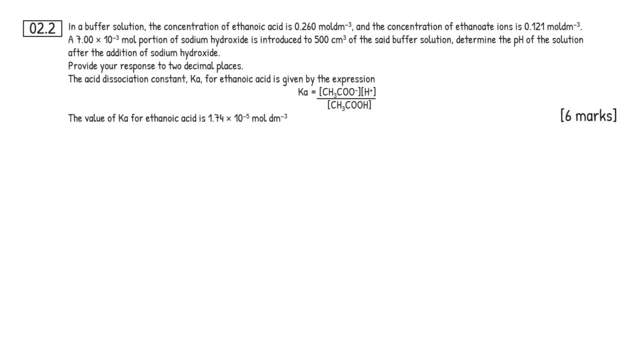 Alright, guys. so this is going to be a buffer calculation question from an AQA A level chemistry pass paper. The paper mark scheme and examiners report will be linked down below in the description. Unfortunately I can't show the actual paper on the screen because of AQA's copyright. but 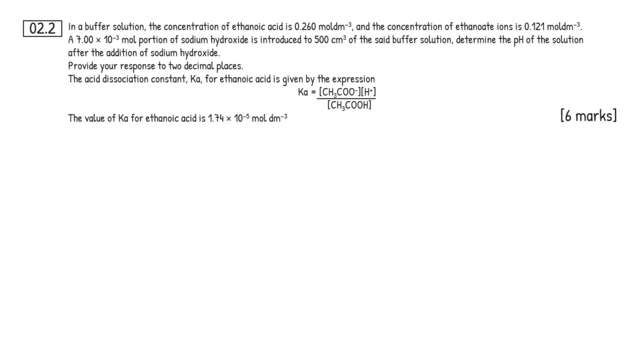 feel free to pause the video, attempt it yourself, see where you went right, where you went wrong and learn from your mistakes. This is key in chemistry. If you want to see more question breakdowns like this, like the video, subscribe all that good stuff. But let's just jump into 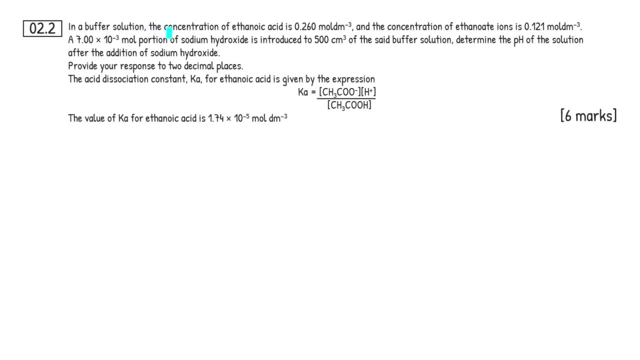 this and read through the question. So in a buffer solution the concentration of ethanoic acid is 0.26 mol per decimetre cubed and the concentration of the salt, the ethanoate ions, is 0.121 mol per decimetre cubed And we have a 7 times 10 to the minus 3 mol portion of 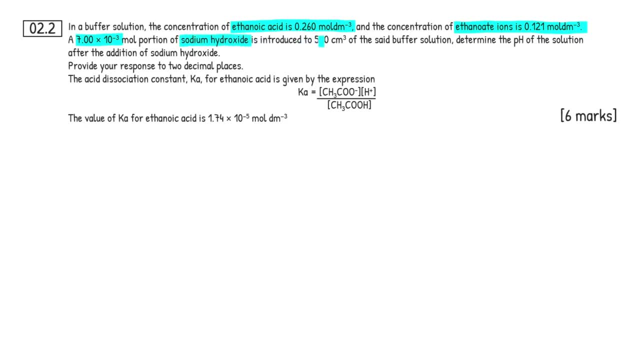 sodium hydroxide. so a strong base is introduced to 500 centimetres cubed of the buffer solution Determine the pH. so that's ultimately what we have to do in the question here of the solution after the addition of sodium hydroxide, And we have to provide our answer to two dps. 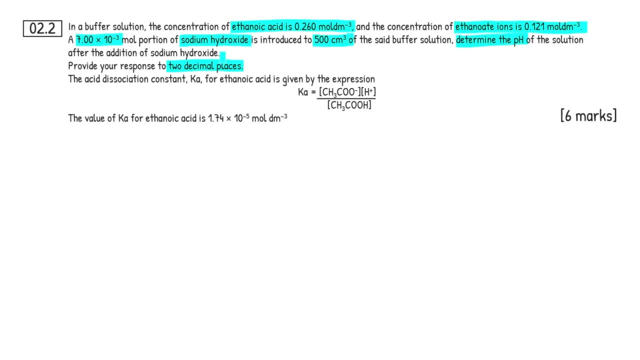 This is never going to change. At A level chemistry, you always want to put your pH to two decimal places. just try and remember that. And I've added this information for the Ka expression and what the Ka value is from the previous question 2.1.. It was quite. 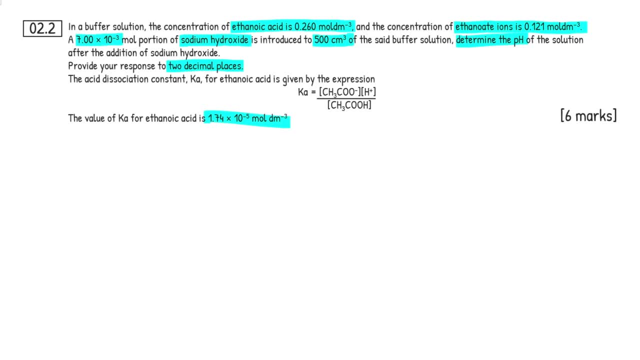 an easy question, so I thought I'd keep it separate entirely. So let's think about buffer calculation for a second. A lot of people, including myself, when I first started doing A levels, I got real confused with what was going on and got a bit overwhelmed. But once you realise the steps involved, it's actually really simple.